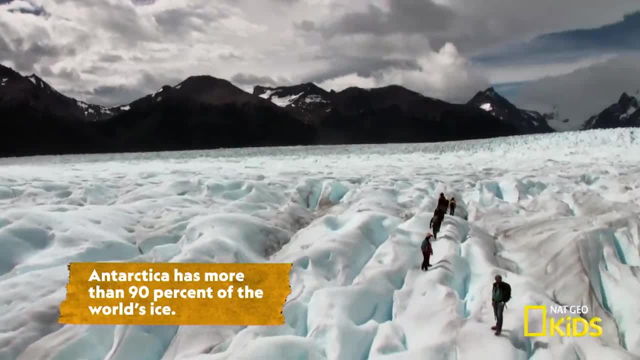 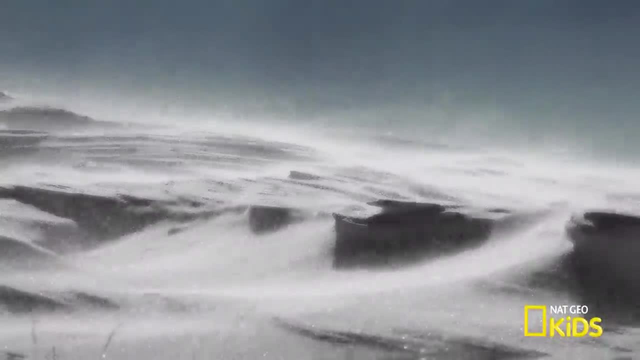 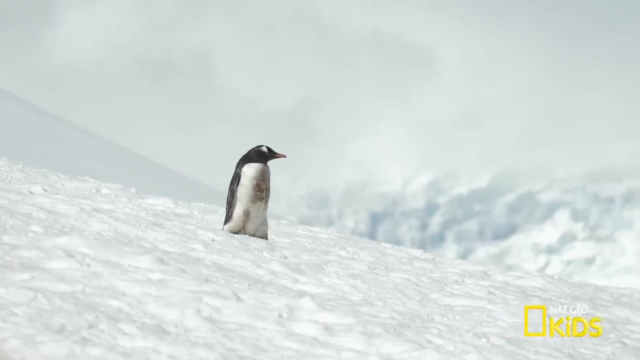 while Antarctica averages just two inches. Instead of the rain soaking into the ground, Arctic rain turns into snow and piles up. Winter temperatures can drop to between 14 and negative 22 degrees, But don't worry, Summer temperatures can warm up to highs around 32 degrees Fahrenheit. 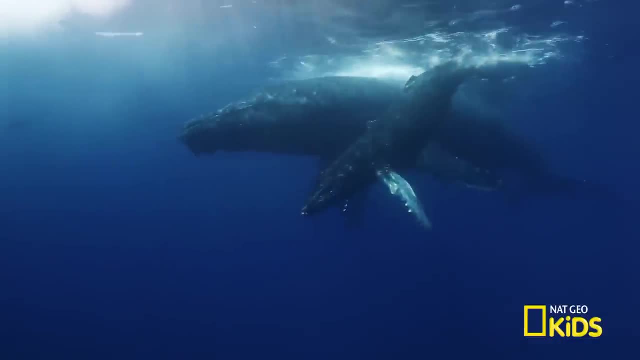 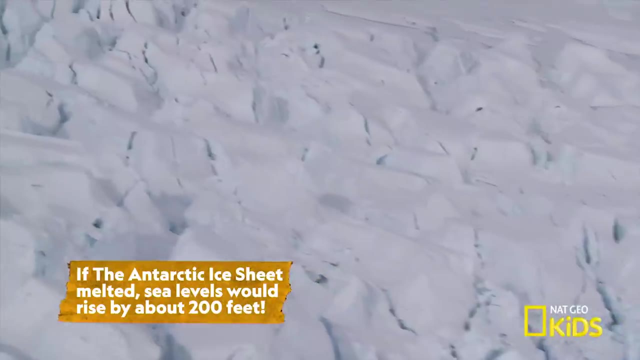 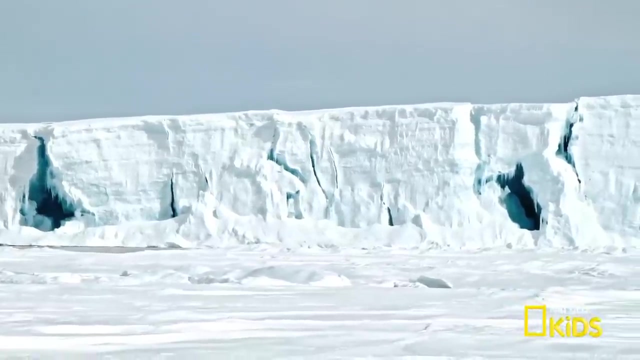 Thousands of tourists travel to Antarctica every year to see amazing animals and more. Let's start with the Antarctic Ice Sheet. It's massive: the largest single piece of ice in the world, covering more than five million square miles. Rising above the ice is the 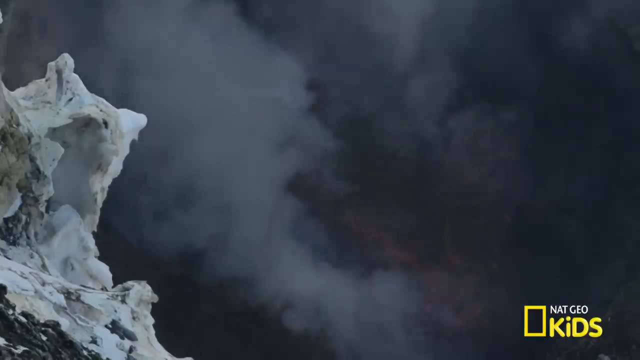 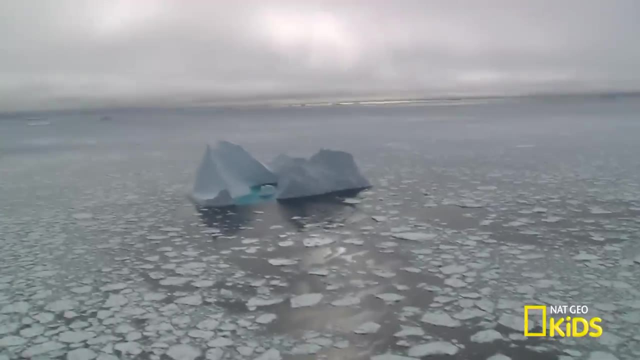 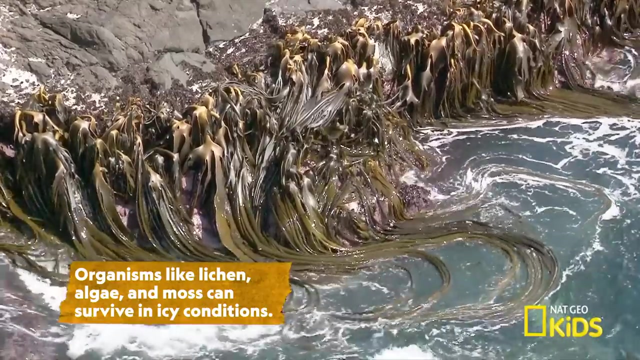 northernmost active volcano in the world, Mount Erebus. Swirling inside the volcano is one of the world's only molten lakes made of lava. Antarctica is a cold and icy place, making it the perfect home for wildlife. Vegetation like lichen, moss and algae have adapted to life above the ice along. 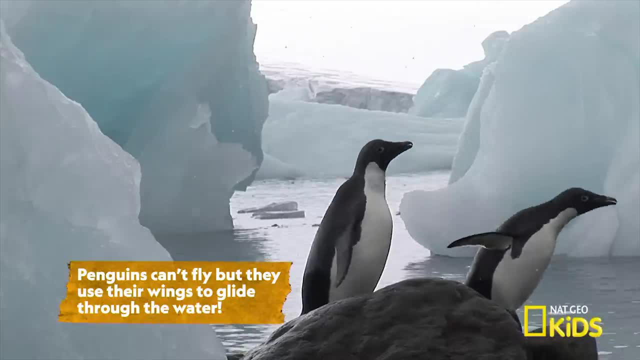 with a few different types of seabirds, including one of the most popular in Antarctica, the penguin, and below The Antarctic Ice Sheet is the most active volcano in the world. It's the most active volcano in Antarctica for precon boarding- withигします. 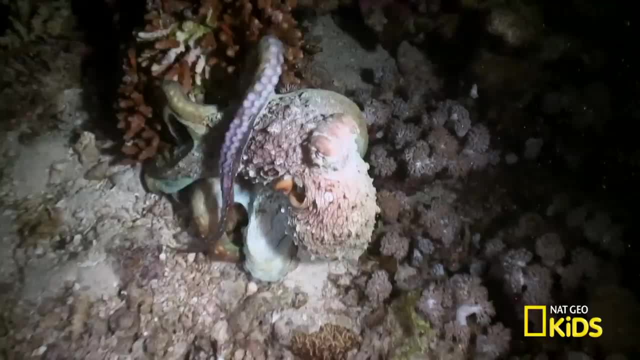 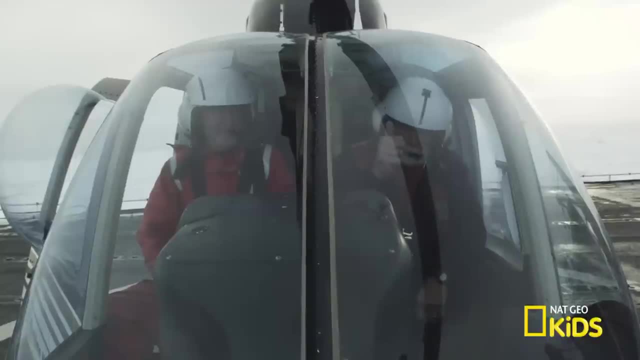 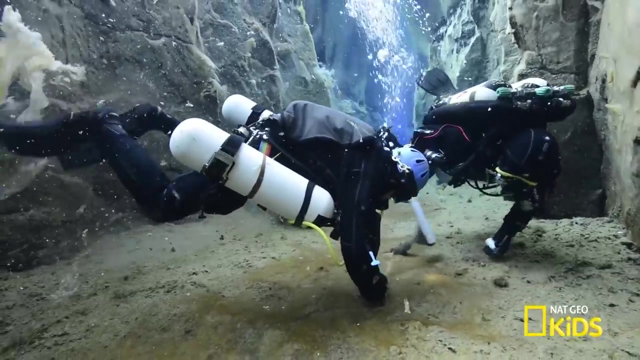 Below the ice are some of the most amazing and diverse marine wildlife on the planet, including seals, octopus and whales, making Antarctica one of the best places for scientific research. Dozens of countries from around the world have set up their own research stations here, studying 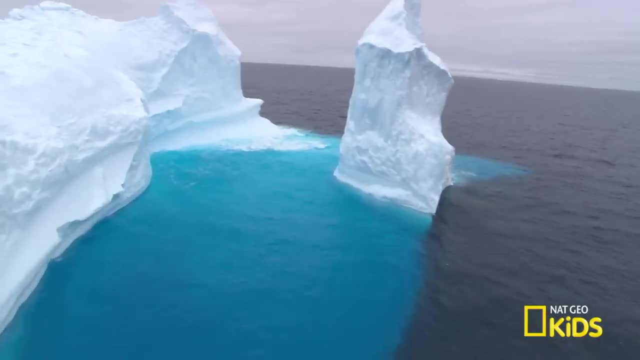 everything from climate change to meteors from outer space. It's the harshest environment on the planet: cold, dry, heat, pH ofés for totalarnos 9енты. dry and barren. But scientists and explorers have been braving this continent. 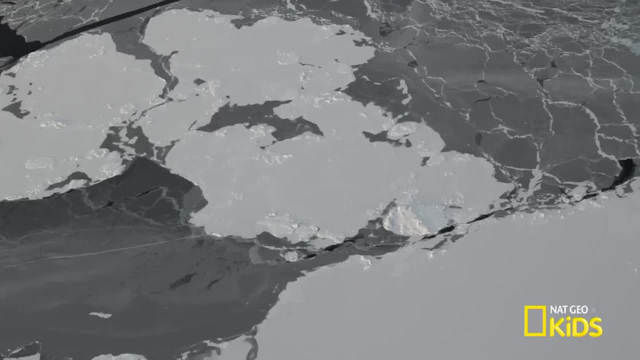 since the early 1900s, And there's still more to discover under the ice and snow of Antarctica, Captioned by Media Access Group at WGBH- accesswgbhorg.